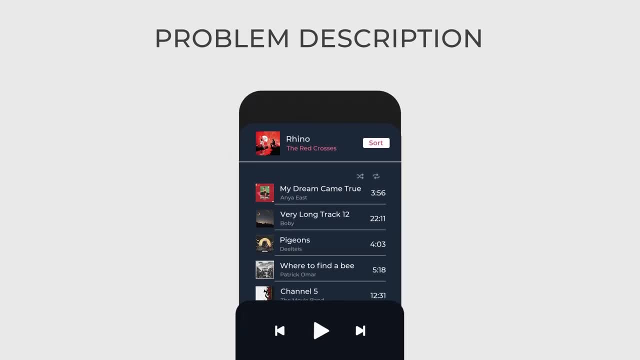 Imagine that you are working on a music application. Your current feature is the next song and, of course, the previous song. In the beginning you thought that this was an easy problem, but you realize that the application's user has several orders to select the songs. 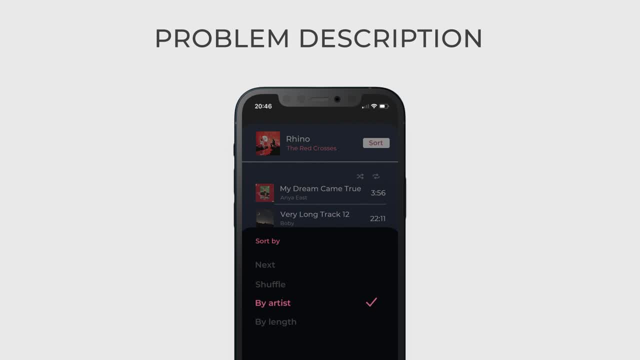 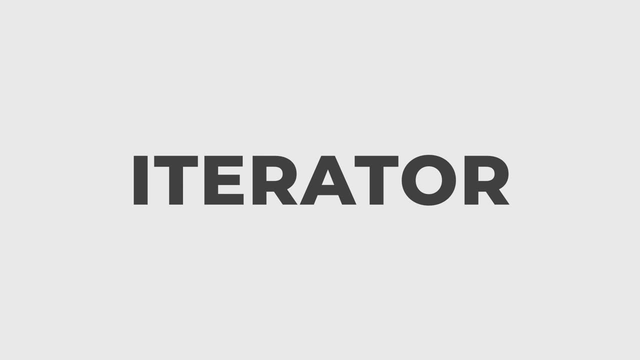 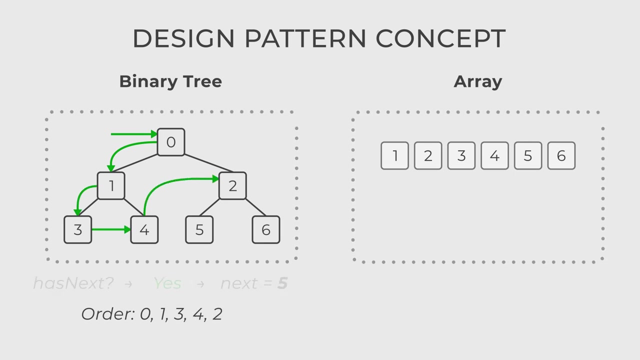 for example, next in list, random, alphabetically sorted, sorted by length, and so on. For this task, the iterator design pattern is the best. The iterator is a behavioral design pattern that provides a way to access elements of a collection without exposing its underlying. 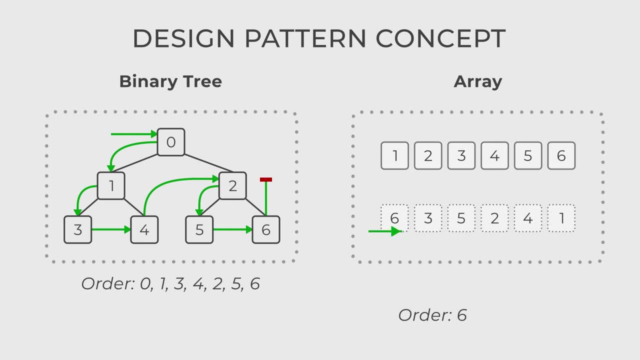 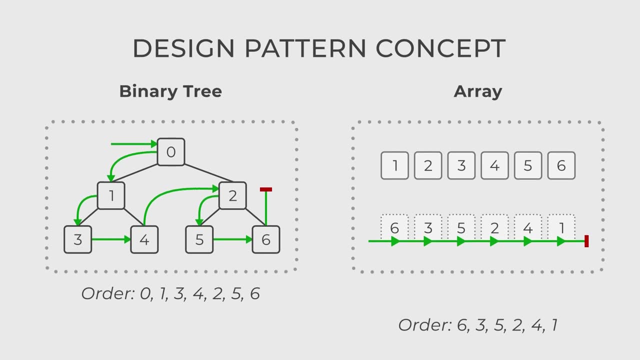 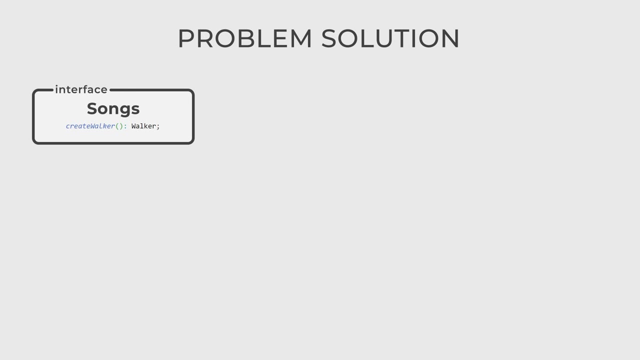 representation. It abstracts the traversal process, allowing clients to navigate through elements sequentially without knowing the details of the collection structure. First, we should have an interface that defines the collection of songs and has the createWalker method. Let's call it just songs. Then let's create the Walker interface with hasNext and 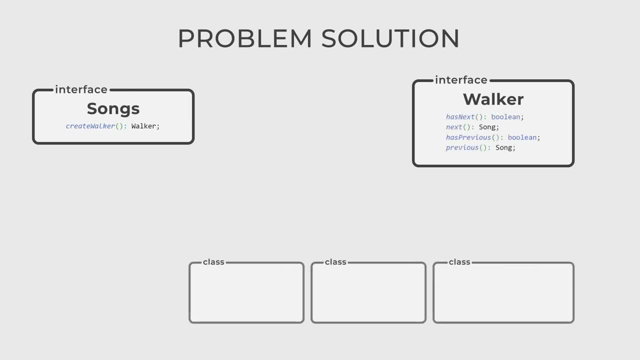 next methods. After that, let's create the concrete walkers Classes that are implementing the walker, for example, randomOrderWalker, simpleOrderWalker and sortedByNameOrderWalker. Each walker knows their specific way to iterate over the song collection. Finally, we can create concrete collections of songs by implementing the songs interface. 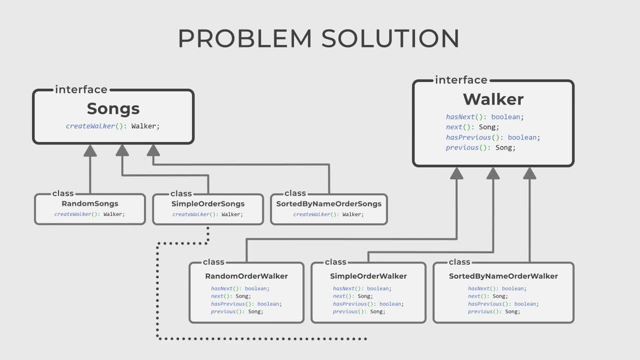 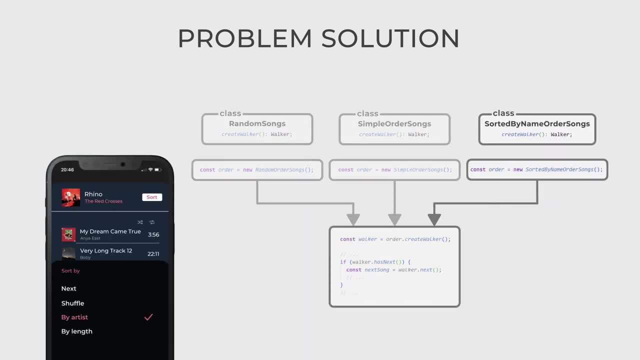 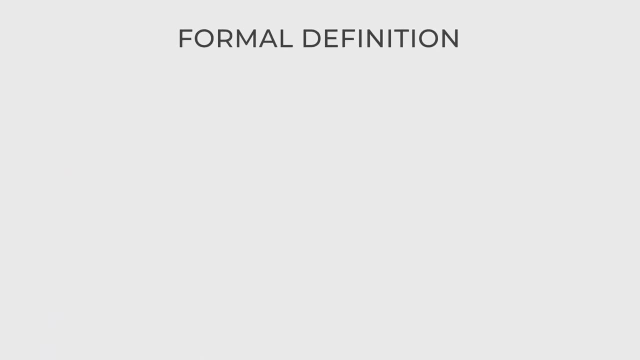 and using the desired iterators: the random songs, the simple order songs and sortedByNameOrder songs. When the user selects their favorite order, you instantiate the appropriate collection and this collection knows how to walk over songs the user has. There are four actors in this pattern. The first one, iterator, is an 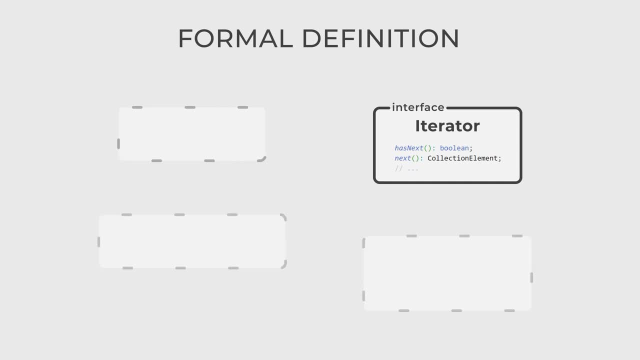 interface that defines the methods for traversing a collection, including operations like next and hasNext. ConcreteIterator is a class that implements the iterator interface and provides the actual traversal logic for a specific collection. Then we have the collection, an interface that defines methods for creating an iterator And, lastly, ConcreteCollection is a class.